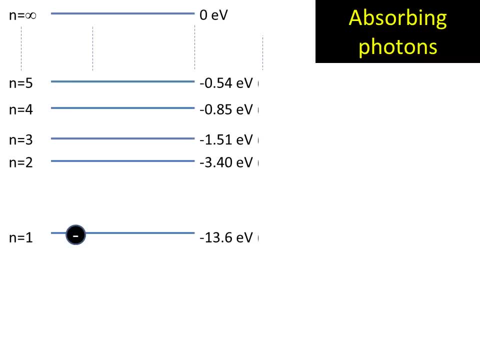 They shoot right out Right now, if I consider I'm going to forget about the nucleus, the proton, because, as I said, this is all about the electron And this is just a little slice, if you like, of those energy levels. 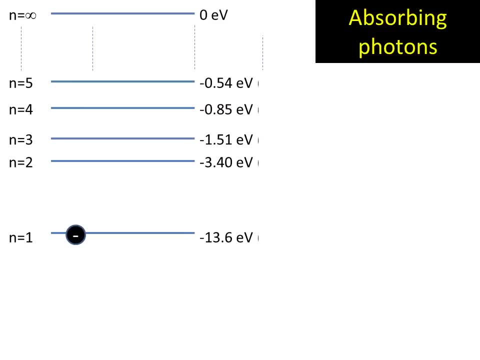 So N equals 1 there ground state, that's where the electron is right now. N equals 2,, 3,, 4,, 5.. And then there's a gap. There are a finite number of these, by the way. 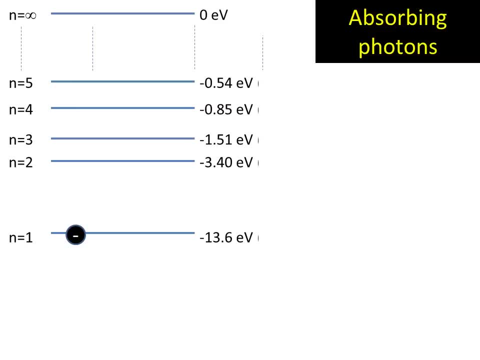 There's not an infinite number- N equals infinity- is just there to indicate that it no longer is under the influence of the nucleus at all. We can see here that it's got minus 13.6 electron volts. Well, I said earlier that this. 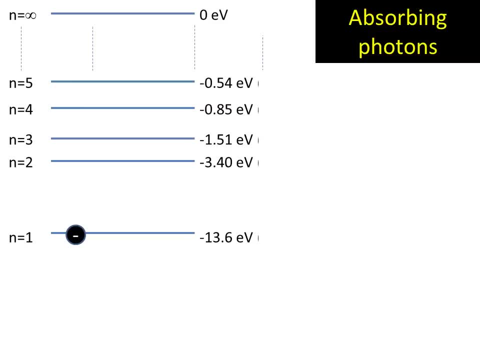 This is at its lowest energy point, And what this tells me is: to get this electron all the way to the ionisation point- N equals infinity- I need to give it at least 13.6 electron volts of energy. Well, let's have a quick look at what that corresponds to in joules. 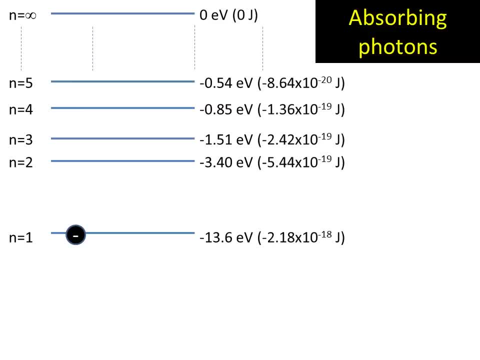 because it's usually easier to think in terms of joules. So here we go. So I've converted the electron volts into joules by simply multiplying by 1.6 times 10 to the minus 19.. And we get this. Well, key bits: 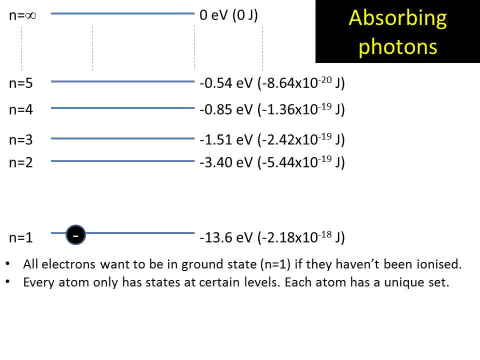 All electrons want to be in ground state. Every atom has certain states, at certain levels, And each atom, Each atom, Every single element, every single atom has a unique set that's unique to it. Electrons have to land exactly on these steps. 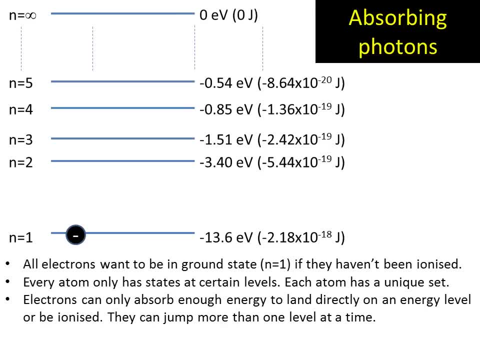 They can jump more than one at a time, but they have to land exactly on them. If they get given energy that's a little bit too much or not quite enough, then they simply ignore that photon totally and it passes them by Okay. 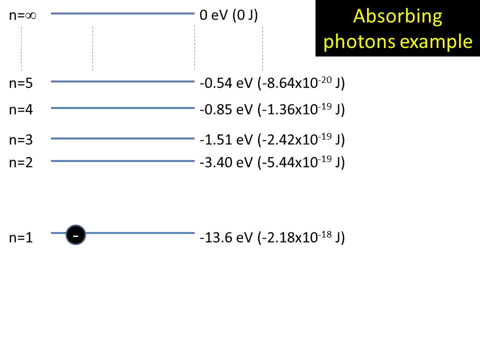 Let's have a quick look at an example for absorbing photons. Okay, so the energy arrives as photons. Here This electron is moving up to to n equals 2. To do that it has to go from 13.6 electron volts to negative 3.4.. 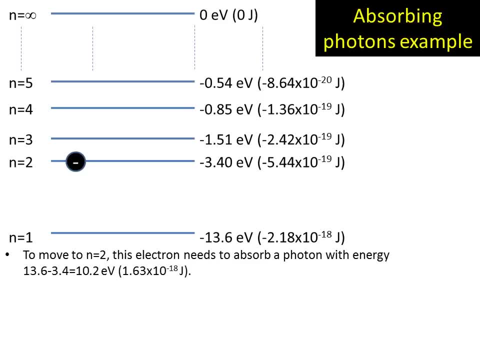 Well, that means a difference. It needs to absorb 10.2 electron volts of energy. If it was 10.4 or 10.3 or 10.19, it would be no good. It simply would ignore that particular photon and it would stay where it was. 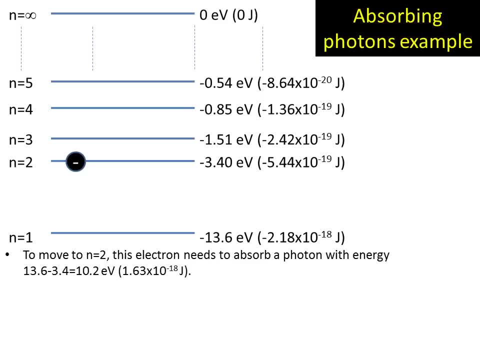 Okay, It can only absorb one photon at a time and it has to be 10.2 electron volts to move that band. If it then got hit by a photon 2.65, then it would absorb 10.2 electron volts of energy. 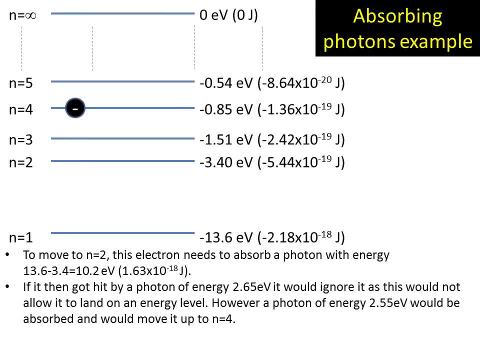 If it then got hit by a photon 2.65, then it would absorb 10.2 electron volts of energy. 2.65 is too big. It misses n equals 4 and it's not enough to get to n equals 5.. 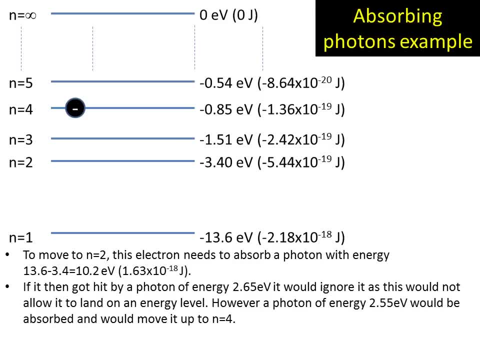 So it has to get 2.55 and it would land then directly on n equals 4.. So it would take that photon and ignore the others. If I was to give it more than 0.85 electron volts right now, it would scoot straight up past n equals infinity and it would be ionized. 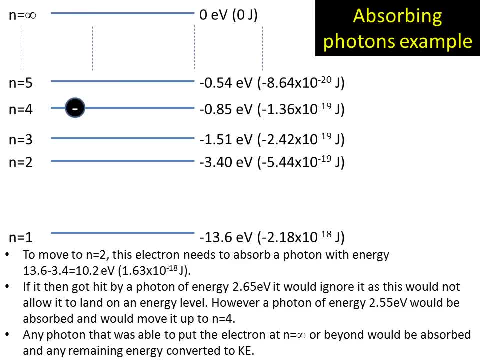 So if I gave it one electron volt, it would use 0.85 of that one to get to ionize and it would then use the remaining 0.15 electron volt So it would be ionized. So it would use 0.85 of that one to get to ionize. 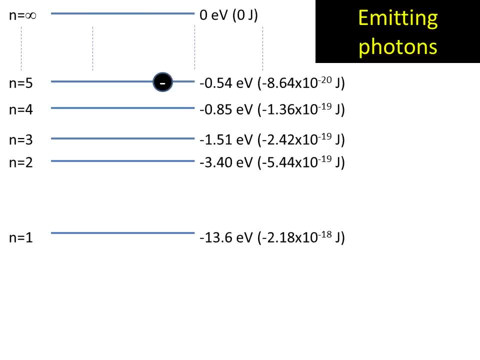 So it would use 0.85 electron volts as kinetic energy by emitting photons. Now this electron is up on n equals 5. It doesn't like to be up there. It wants to get rid of energy. It wants to get down to n equals 1, down to ground state. 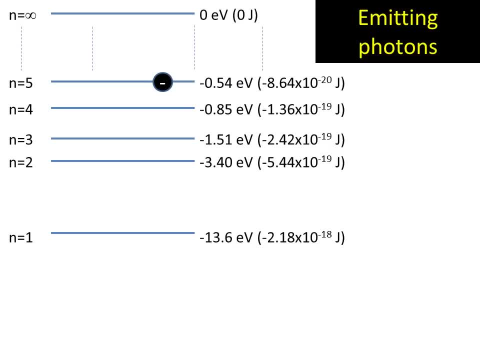 The only way it can do that is by emitting photons. So this particular electron wants to get down there and the only option it's got is to jump down energy levels. It doesn't have to jump one at a time. It could jump straight from n equals 5 to n equals 1.. 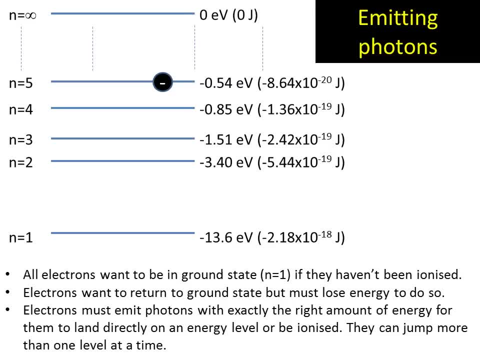 It could go from 5 to 3.. It could go from 5 to 2 to 1.. It doesn't matter how many steps it takes, But by getting rid of only certain, There's only a certain combination that it can follow. 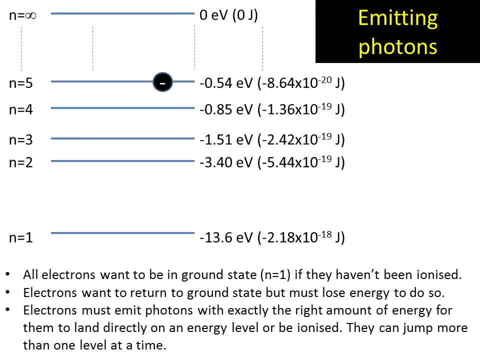 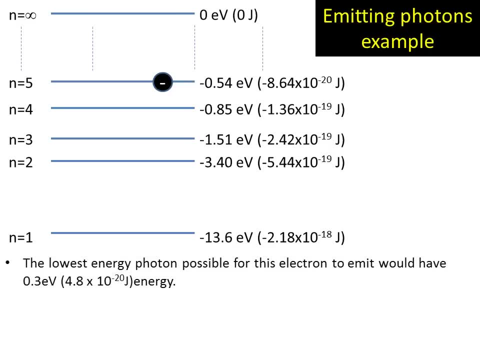 There isn't an infinite number, which means there are only certain photons it can release, And certain photons mean certain colors. So let's look at an example here. So the lowest energy possible for this one, the smallest amount of energy it can possibly lose. 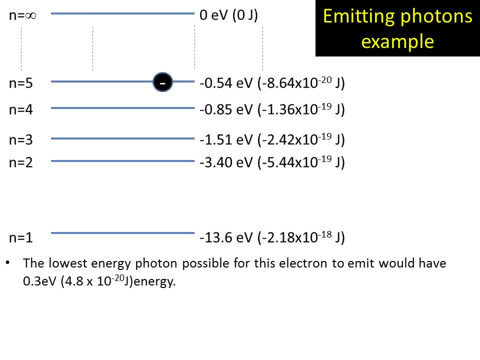 would be to move from n equals 5 to n equals 4.. So band 5 to band 4, which corresponds to a loss in energy of 0.3 electron volts. That's the smallest, the lowest energy photon this electron could ever emit. 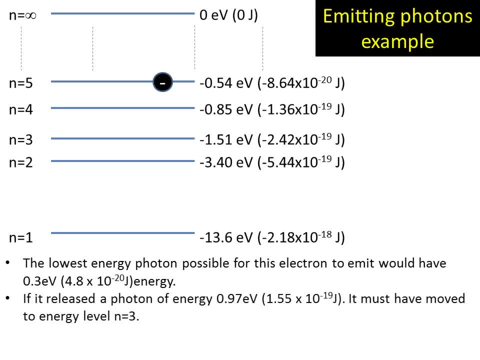 Okay If it released. so if we measured it in a photon and released it and it came out as 0.97, we could actually work out that it must have moved to band 3 because the difference between 0.54 electron volts